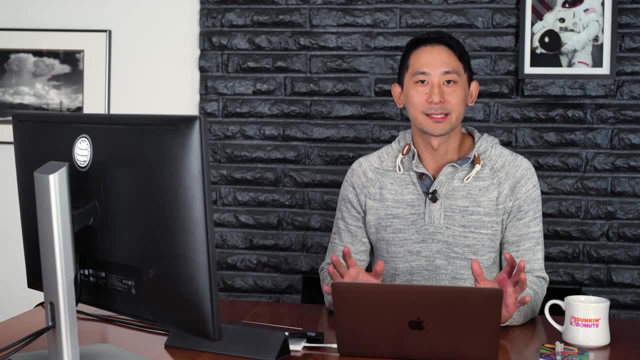 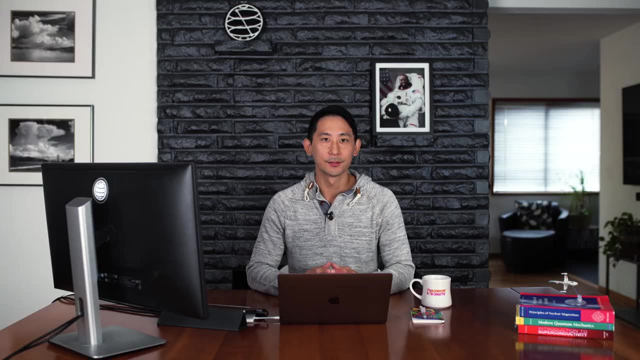 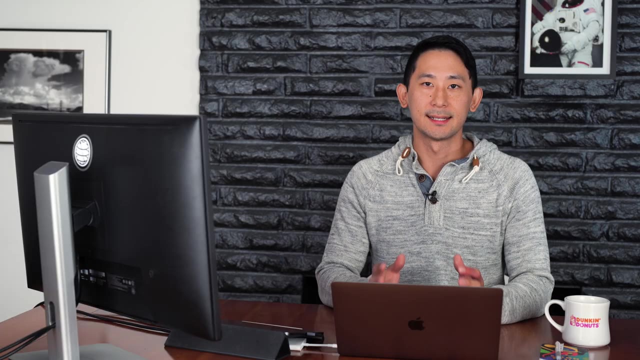 all four of my constraints. By encoding my constraints into a quantum oracle, I could theoretically figure out which restaurant I should order from faster than if I were using a classical computer. For a reasonable number of restaurants, my phone can do this just fine. But what if we're thinking about big datasets? For big datasets we can have. 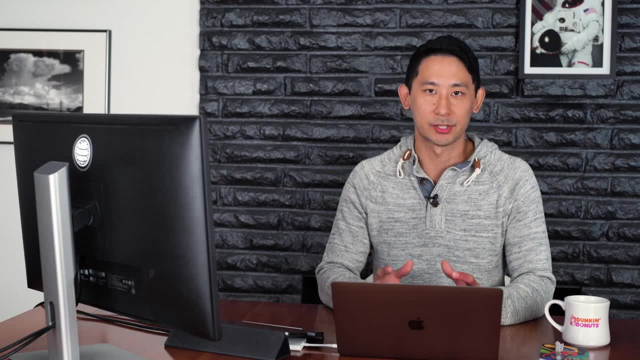 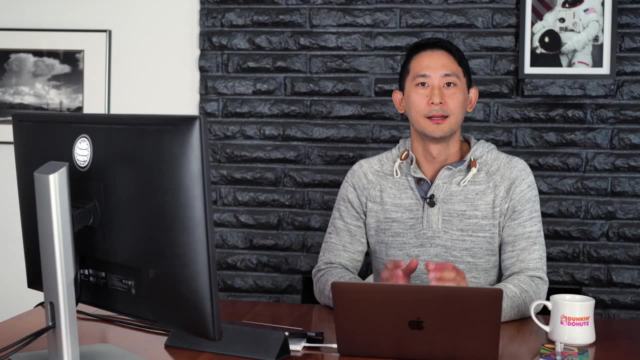 a quantum speedup because we can recast this problem into a search problem. We can search over every combination of inputs and determine which input evaluates to true given our constraints. Another useful example of a Satisfiability Problem that we're going to implement today: 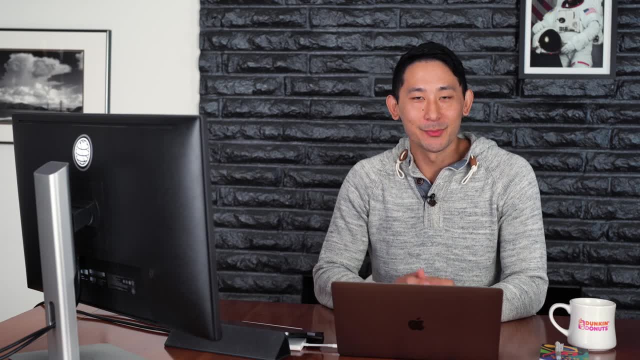 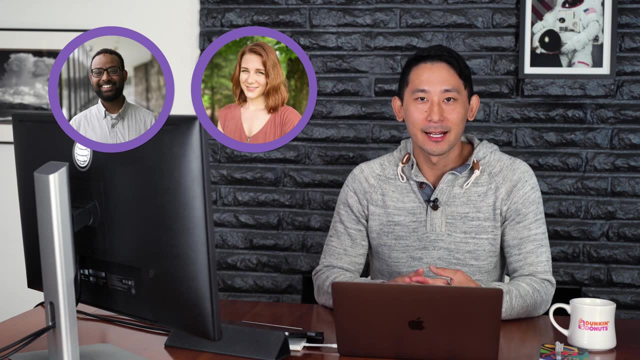 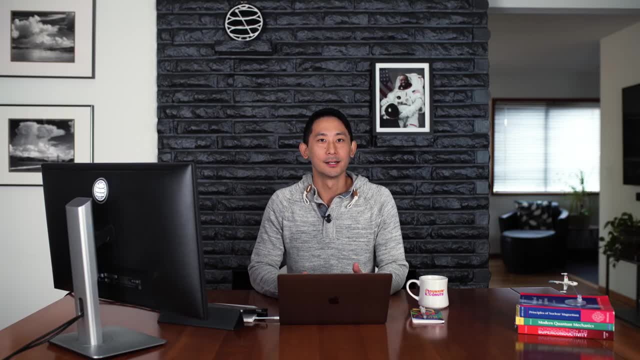 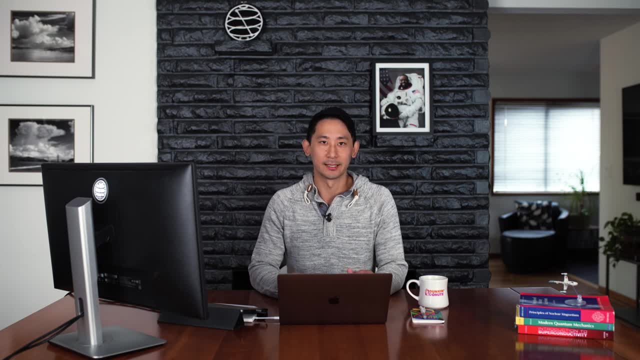 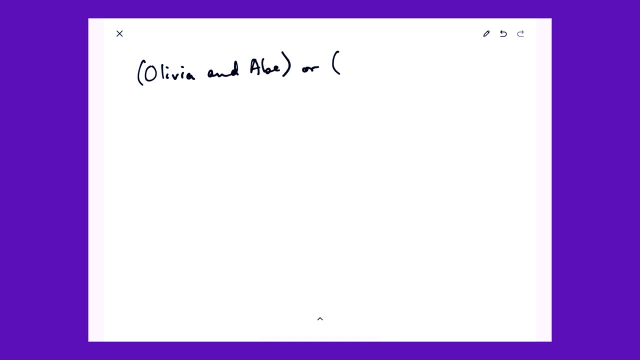 for our party planning problem can be formulated with the following Boolean expression: So we can have Olivia and Abe or Jin and Amira and not Abe and Amira. And we can simplify this a little bit just by saying A and B or C and D and not A and. 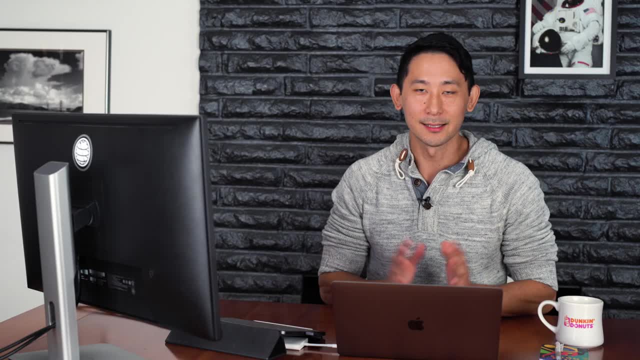 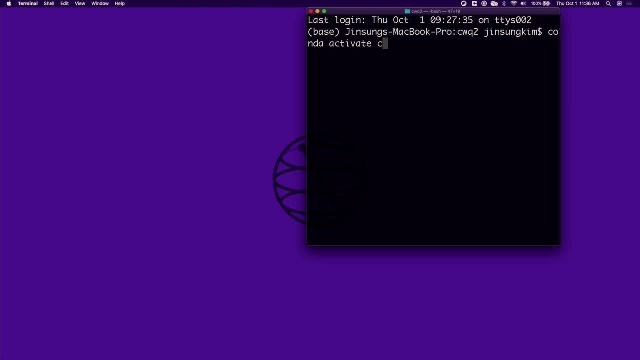 D. So let's see what this looks like in Qiskit. So I'm going to first activate my environment going with Qiskit. There's where I have Qiskit installed and I'm going to open up a Jupyter notebook. 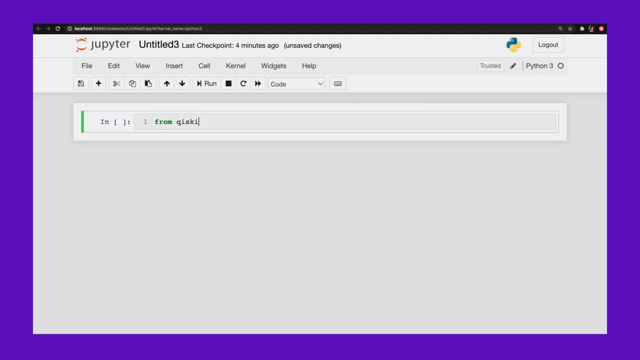 So from Qiskit I'm going to import my simulator, Basic Air. From Qiskit aqua algorithms: import my Grover search. From qiskitaqua componentsoracles import my oracle. Okay. From Qiskit tools visualization, import plot histogram so I can see my results. 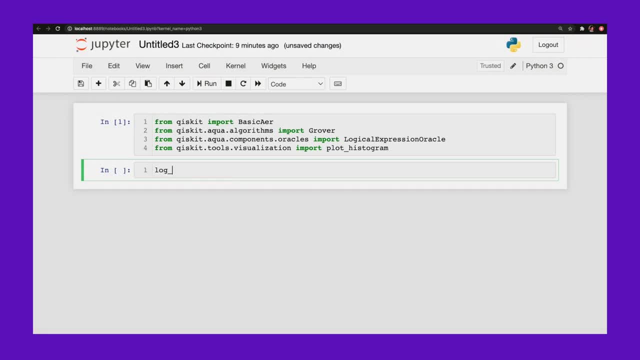 So I'm going to encode my logical expression in here. so it's going to be Olivia and Abe, or Jin and Amira, Okay, So I'm going to encode my logical expression in here. So it's going to be Olivia and Abe. 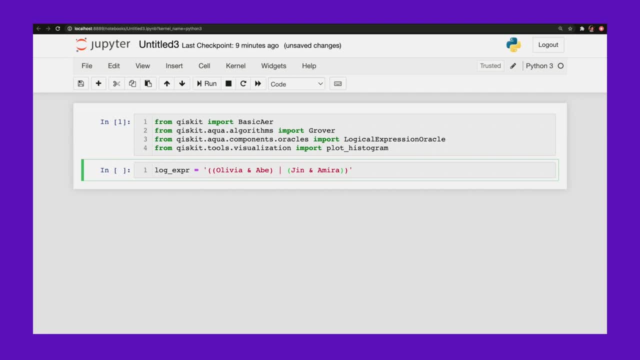 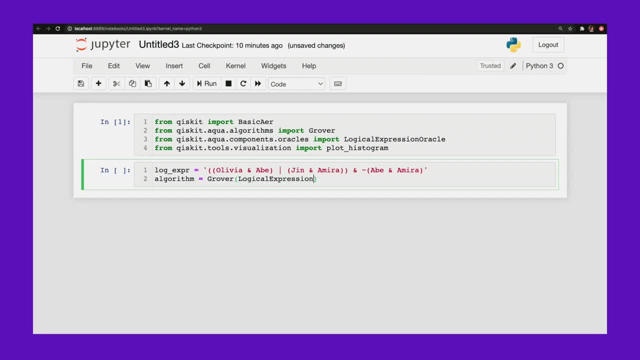 Which is my Grover search Logical expression. Oracle Plug in my logical expression expression: Okay, good, I'm going to get my back end, So I'm going to grab the basic error simulator, from which I'll grab the chasm simulator. 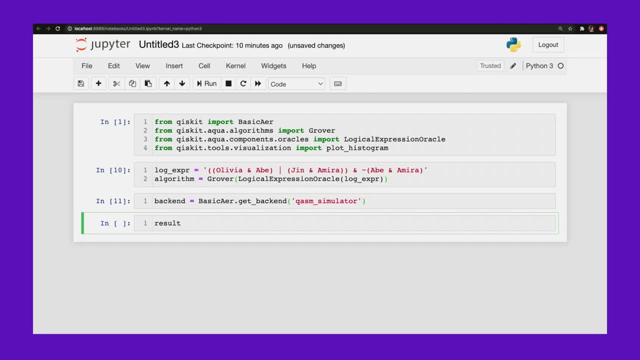 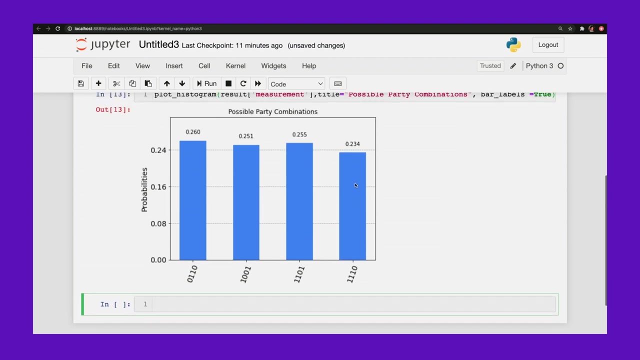 Okay, good. Now let's run this algorithm. Okay, good, All right, let's plot our results, The measurement results, Possible party combinations, Our labels: is true- Okay, good. So what we're seeing here is the possible combinations of people I can invite to. 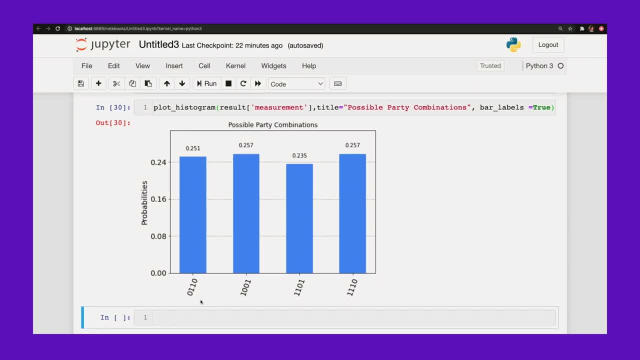 the party. So each number represents whether or not each person should be invited or not, And these are organized alphabetically. So this will go: Abe, Amira, Jin, Olivia. So one possible combination is: Amira and Jin are invited. That's what this first column is saying.